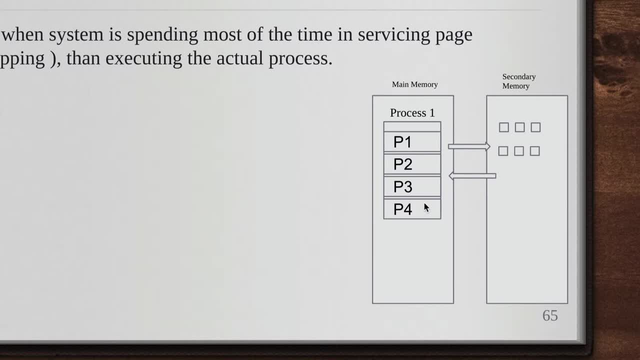 instance it requires: if it requires page five, then page four is going to be swapped, And or if it requires, let's say, page five, So for instance, page one is going to be swapped, it goes to the secondary memory and the page five comes into the main memory. Okay, 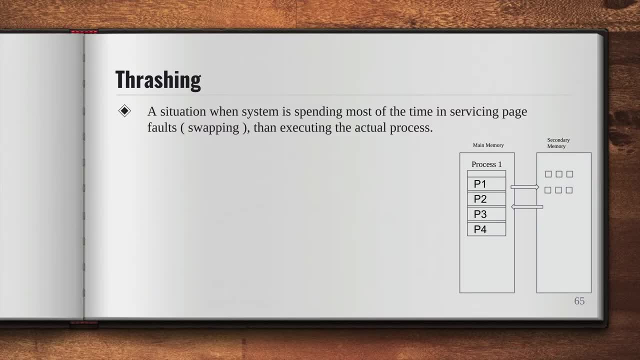 So when does it happen? When does the thrashing happens? So if a process is allocated too few frames, then they will be too frequent page faults And, as a result, no useful work would be done by the CPU and CPU utilization will fall drastically. And this drastic fall of the CPU utilization is called 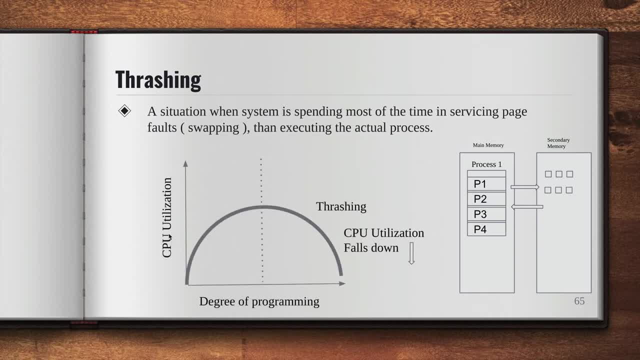 thrashing. So let me show you. So let's say, in this diagram we have the CPU utilization which goes up in this direction, And then we have a degree of programming. So degree of programming means the number of processes at a particular time. So if we are saying, increase the degree of 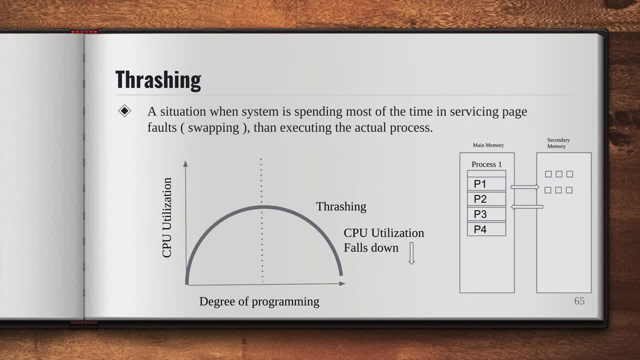 programming means increase the number of process. just a concept, okay. So the CPU should have as many processes as possible so that the degree of programming is high and our CPU is utilized fully and it's not sitting idle, right. So that is why, from here, if you look at the graph, this: 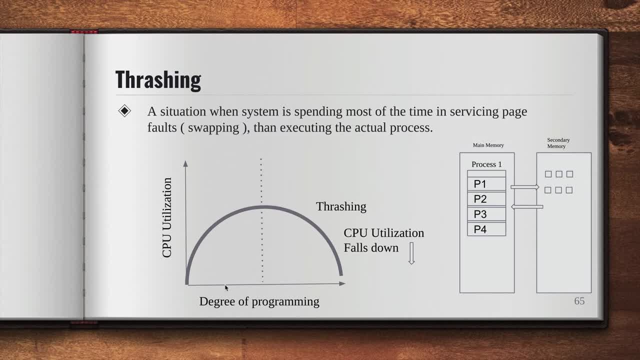 is a utilization. this is the degree of programming, which means when the degree of programming increases- number of processes- the degree of programming increases. So that's why we have the degree of programming increases. So that's why we have the degree of programming increases. So that's why we have 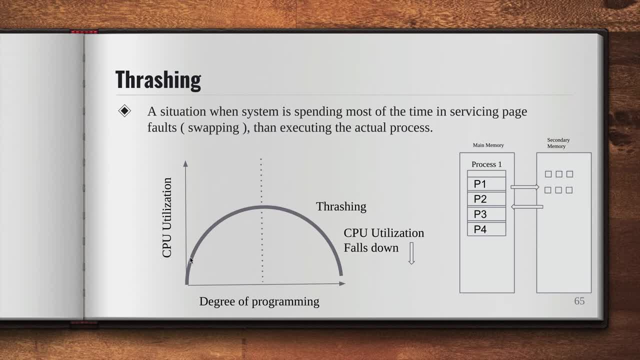 increases in the CPU, then the CPU utilization increases. So like this it goes up like: but at this point there will be, there will be a point that will come And at that stage probably there won't be enough frames available. So the swapping would happen. And as soon as the swapping happens, 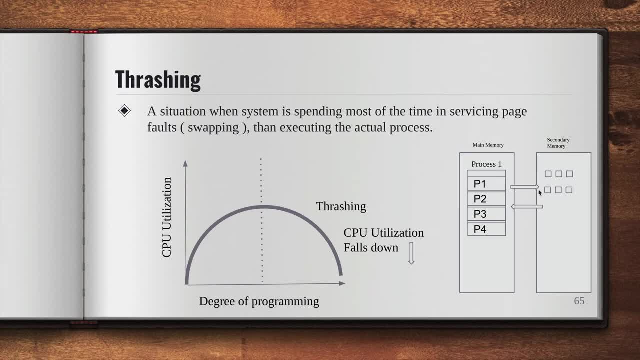 CPU will become busy in getting those pages rather than doing the actual task And from this point onwards, the CPU utilization will fall down is because the CPU is busy for doing the swapping of the pages rather than doing the axle task. Okay, so at this point, operating. 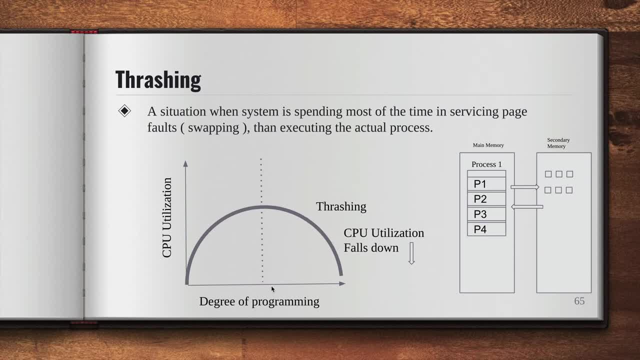 system would think that it needs to increase the degree of programming, so it will start increasing the number of processes. That means that the long term scheduler would try to load more processes into the main memory to improve the CPU utilization. But the problem is that this will result in